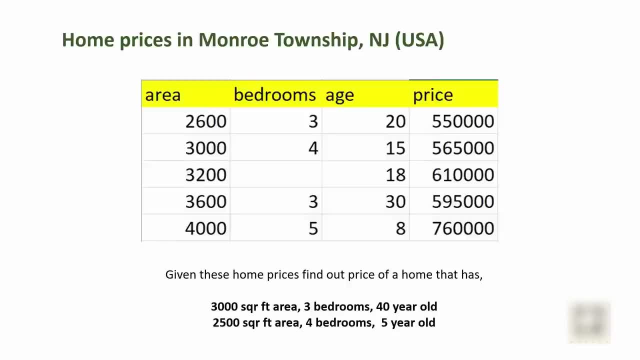 We need to carefully analyze our data set or our training data. When I look at this data set, the first thing I notice is there is a data point missing here, so we have to do something to handle this missing data point. Another thing that I notice is there is a linear relationship between 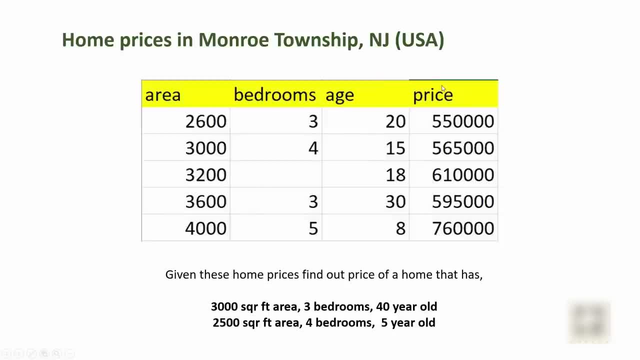 each of these factors and our target variable, which is price. For example, as the home gets older, the price tends to go down. Here I have 3200 square feet home with 18 years of age and the price is more than 600 000, whereas I have a little bigger home here, 3600 square feet- but since the age 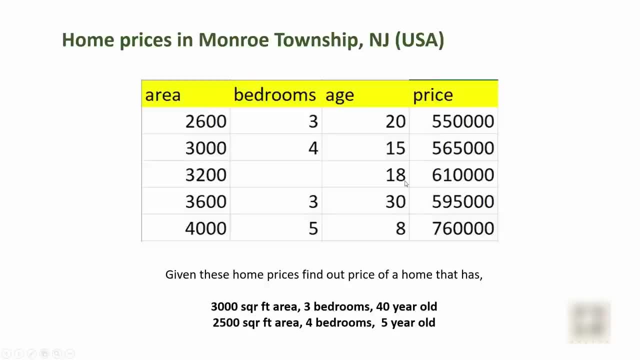 is more, the price is less than the one whose square foot area is less. okay. Similarly, as the area and number of bedroom goes up, the price also tend to go up. So overall, by analysis, we can say that for this data set we can use linear regression safely okay. If we go into a math a little bit, then our 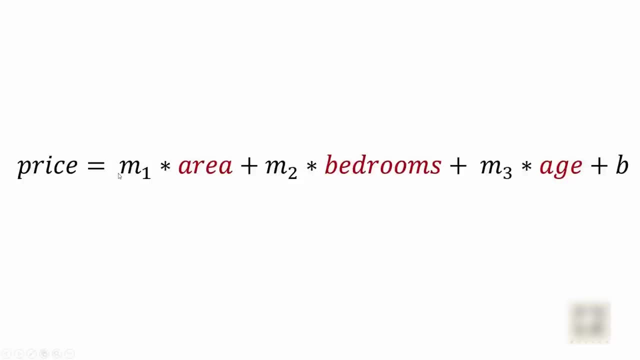 linear equation will look something like this, where price is dependent on three factors- area, bedroom, age- and these three factors are called independent variables or features. Features is a term that you will hear often while going through machine learning material. It is nothing but an independent variable and the price is a dependent variable. M1, M2 and M3 are called coefficients. 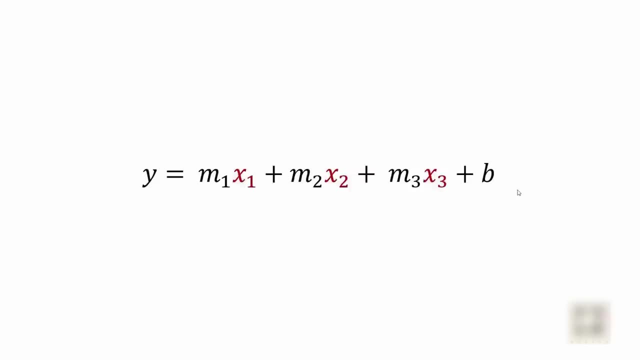 and b is an intercept. It can be generalized into this equation where you can have n number of independent variables. I just have three here, but you can have more than three. Now, the topics that we are going to cover during this tutorial is: first, we'll look into how to handle that missing. 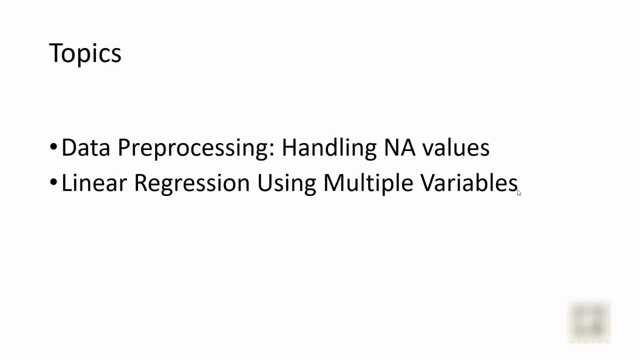 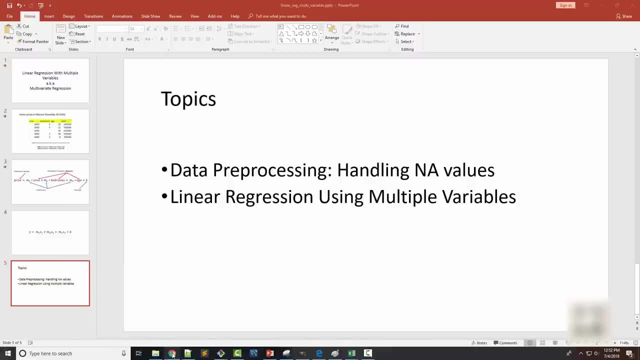 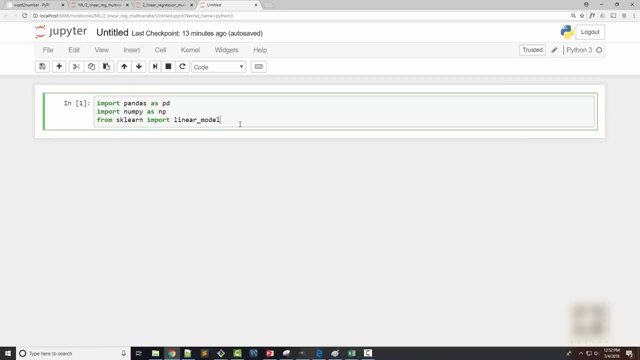 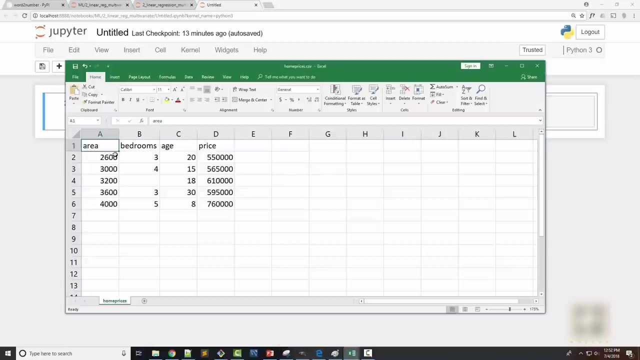 data point and then I will build a model in a python code. All right, now let's go back to our jupyter notebook. So jupyter notebook is something I'm using to write my code. You can use pycharm or any other IDE of your choice. I have a csv file here where I have all my home. 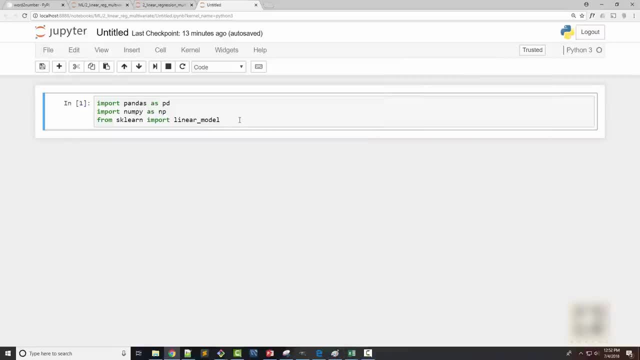 prices, data frame, along with these factors. So the first thing I have done here is imported unnecessary modules and then I am going to load my data into pandas data frame- homepricescsv. If you don't know about pandas data frame, then I have a separate pandas tutorial. 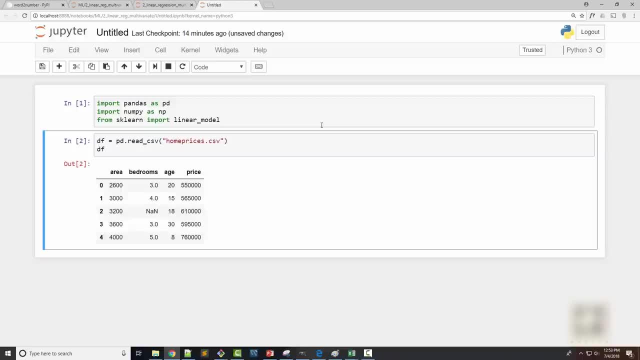 Pandas is extremely useful while doing machine learning. So if you don't know about it already, Okay, so now I have my data frame ready and I can see this null data point and I need to handle it. So the way I'm thinking I will handle this is: I will take 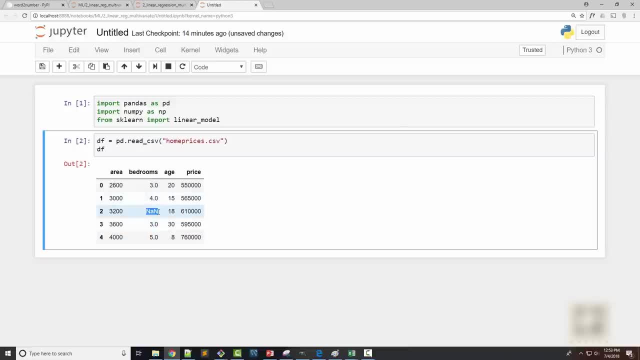 a median of this entire column and put it here. Since number of bedrooms are missing, taking median seems like a safe assumption, All right, so first thing I will do here is calculate the median. How do you calculate the median of bedrooms? So dfbedrooms will give you pandas series. 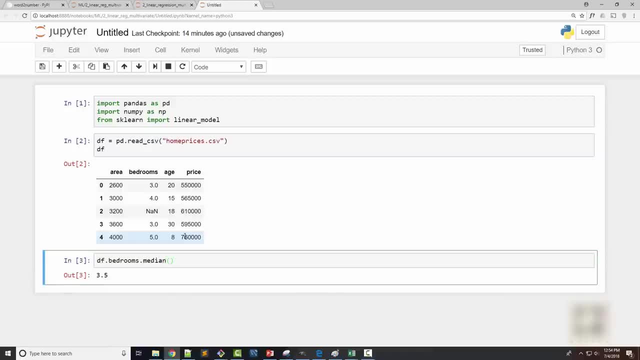 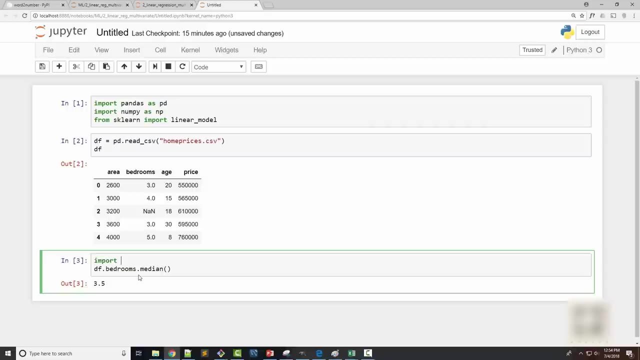 and when you do this it gives you a median. Now you have three bedrooms appearing two times. that's why it's giving the average of it, which is 3.5.. I just want to keep it, integer the whole number, and for that I will just import a math module. 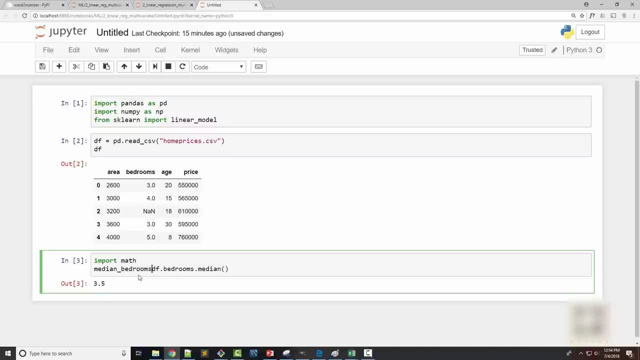 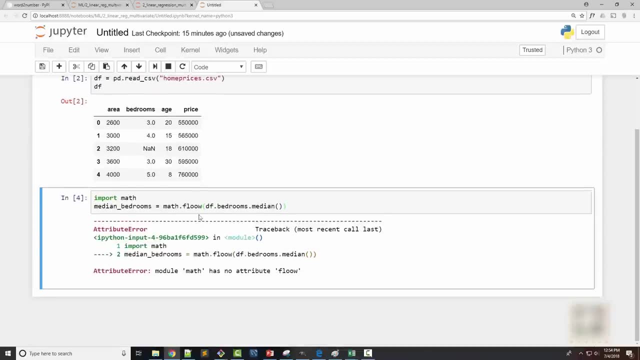 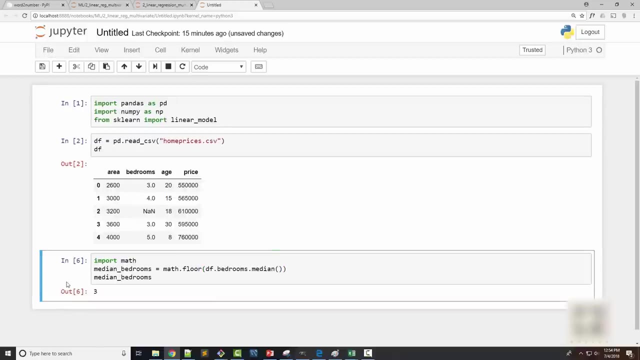 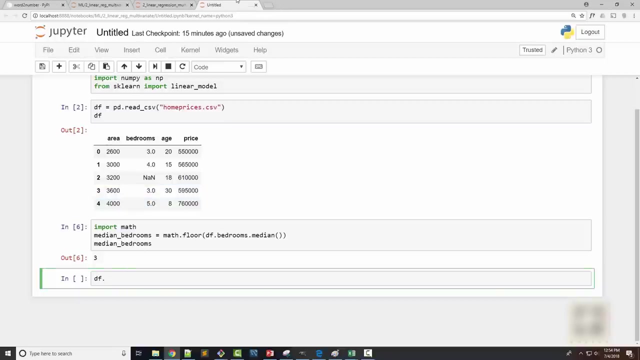 and I will say median Bedrooms is equal to matfloor and the median bedrooms would be 3.. Okay, and the way I fill this columns n a, values, is using FillNFun. The FillNF function is available on pandas series, So dfbedrooms. 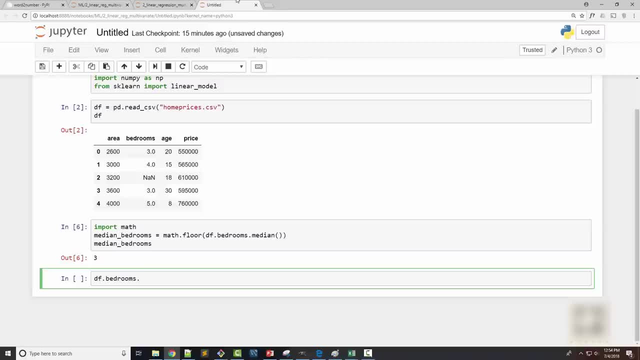 will give you where theUA anda will be. here You are going to get 2.20Nstandard言 you one column which is nothing but a panda series. on that i call fill any function and i want to fill all any values with this median number. so you can see that i got a new series. 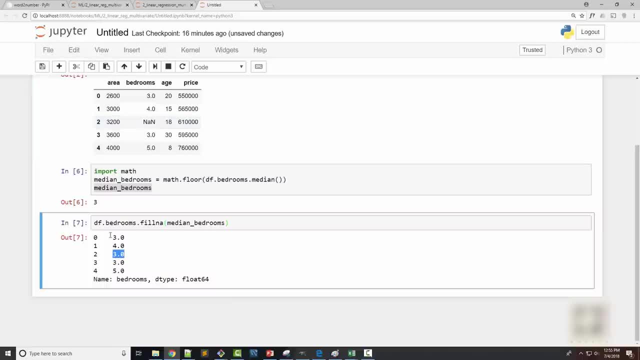 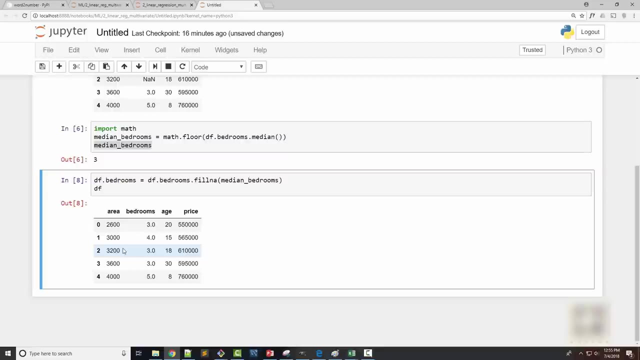 where this nn value is now replaced with a median number, i need to assign this back to original series so that my data frame gets updated and when i print my data frame i can see my data frame looks much better. so our data pre-processing step is over. so again to summarize before applying: 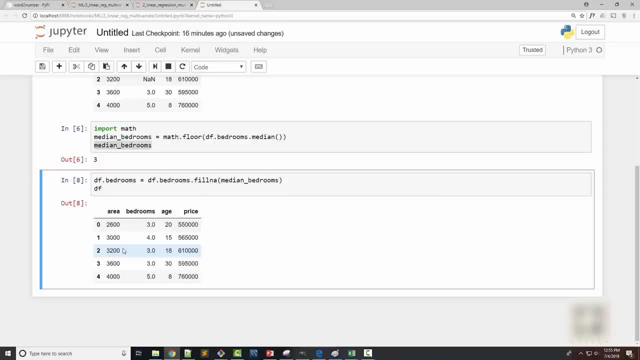 any machine learning model, you need to pre-process your data, you need to clean your data, because data is always messy, there are problems with it, so you need to fix the errors, kind of prepare your data and then apply your actual machine learning model. using that data, you train the model okay. 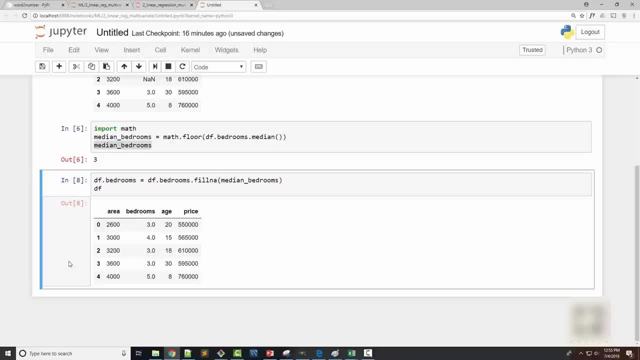 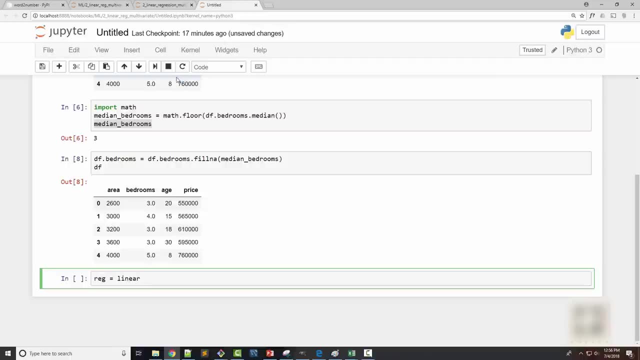 so now my data frame looks good. i am all set to train my model. so the first thing i am going to do is create a linear regression object. so i have imported linear model here and using this i will create linear regression class object. the object got created. fine, now i will call fit method. so you will use this fit method often. 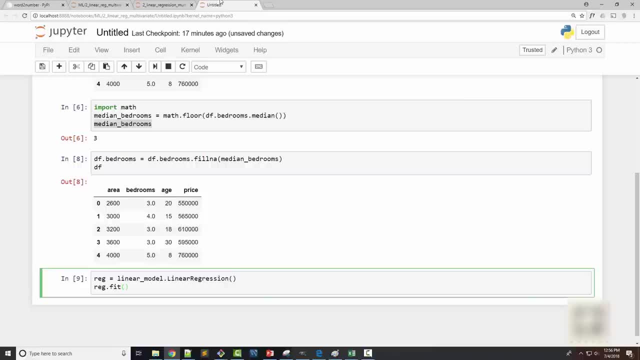 and this method is used to train your model using your training set. here my training set is a data frame, so if you want to create a data frame using your existing data frame, you can use this syntax of using two, two brackets. okay, and my independent variables are area. 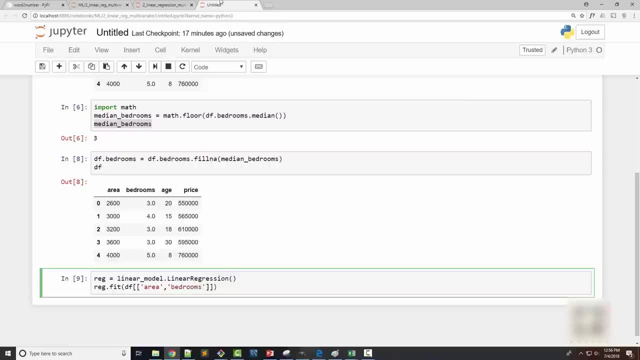 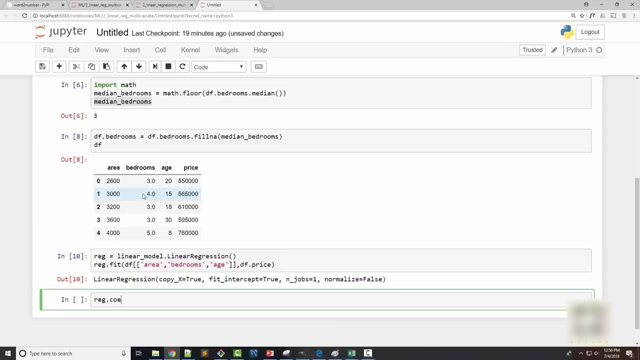 bedroom and age, and my target variable is price. when i execute this, my model is now ready. once it is ready, it's a good idea to take a look at the coefficients. so the coefficients i got was 30 percent and the number of percent is 2.5. 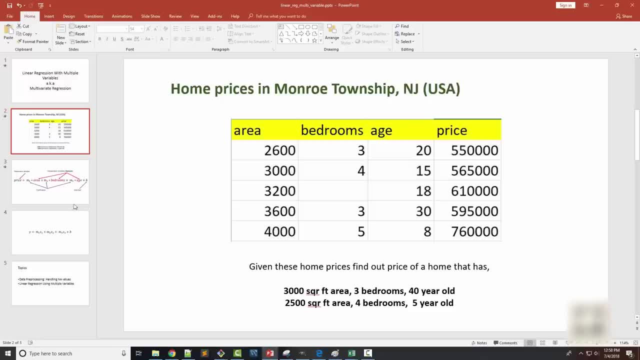 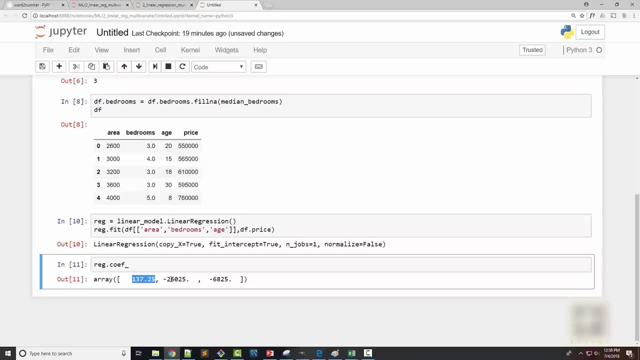 this. uh, just to summarize what these coefficients are in this equation, m1, m2 and m3 are coefficients. so this is m1, this is m2 and this is m3. now you'll wonder: where is my intercept? intercept is stored in another variable called intercept. 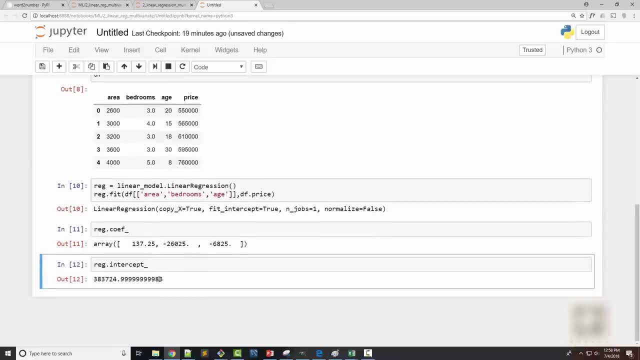 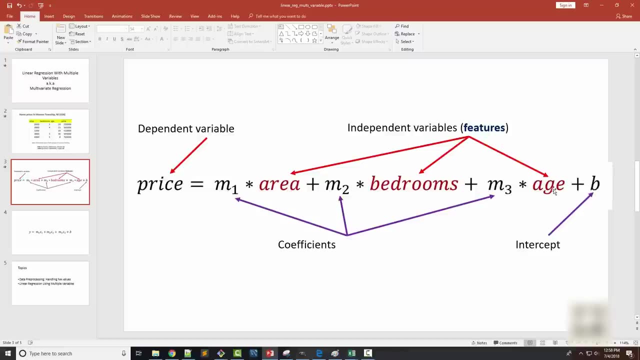 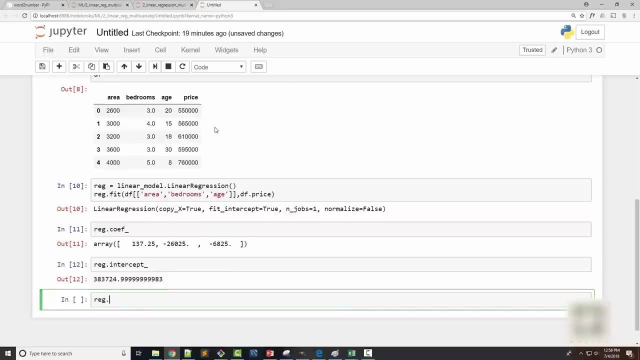 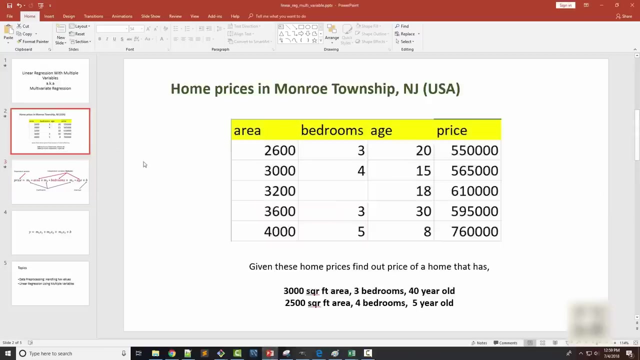 so this number is this b. so once we have m1, m2, m3, you have area, bedrooms, age, which are your independent variable. now you can calculate the price. so here i can say predict, okay, so i can predict a home price of a home whose dimensions are this: so 300, 3 000 square foot, three bedroom and 40 year old. okay, 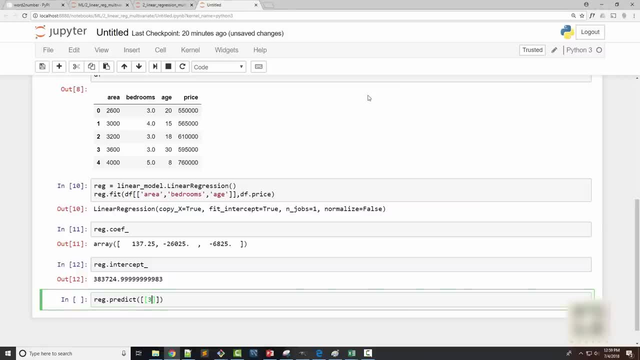 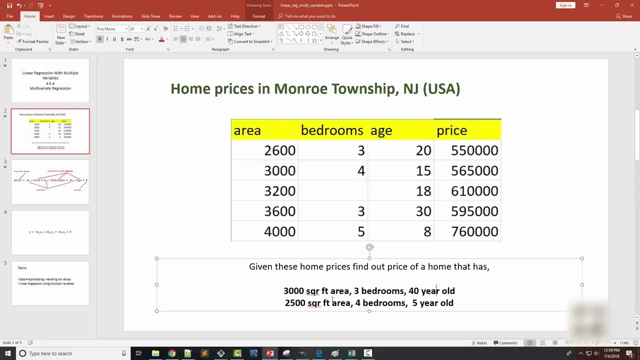 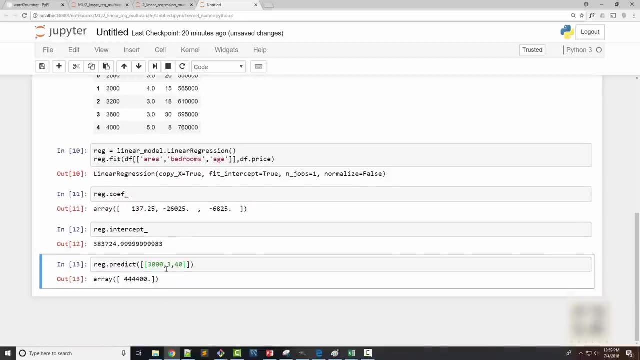 so three thousand three and forty, that's what i'm going to supply here. three thousand three and forty and, if okay, so three thousand square foot, three bedroom, forty year old, and i found find the price to be this much. all right. so this home is, you can see that, the price. so the price of the 3000 square foot home here is 565 000, but here got it. you got it much less and the reason is, i think, mainly age. so here it is like 40 year old versus this home is 15 year. 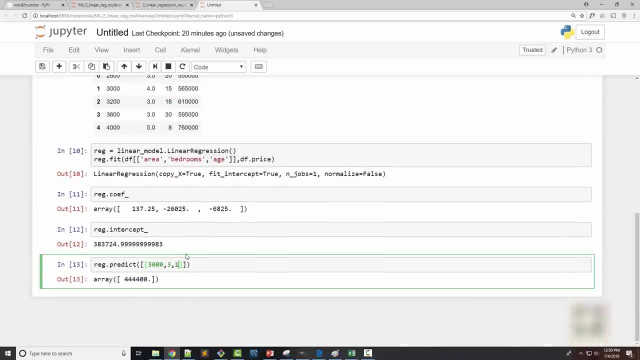 old. okay, so if i make it 15 year, i will get around the. it is little bit skewed, but you get the ballpark all right. so the price is this, and now i want to know how it calculated this price. so it is coefficient, okay, coefficient multiplied by your square foot, plus another coefficient. 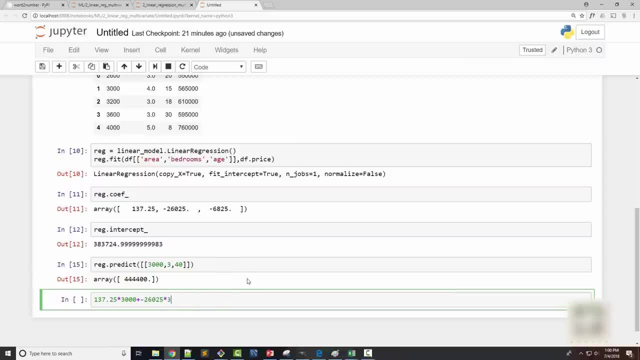 multiplied by your bedrooms. the third coefficient multiplied by the age. here it is missing an intercept, so we need to add intercept also. so plus intercept, and when you do that you get that price right here because of rounding factor it's not showing the full value, but it is essentially the same price. similarly, you can predict: 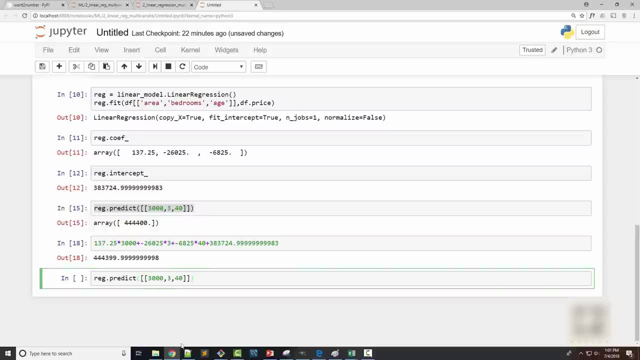 the price of the home and you can also do buying and selling, which is where the value of those factors is 2500, 4 and 5 500 anywhere. 주인이: this home is very new, so i expect the price to be a little higher than average. so here you can see that 58 588 000 is the price. 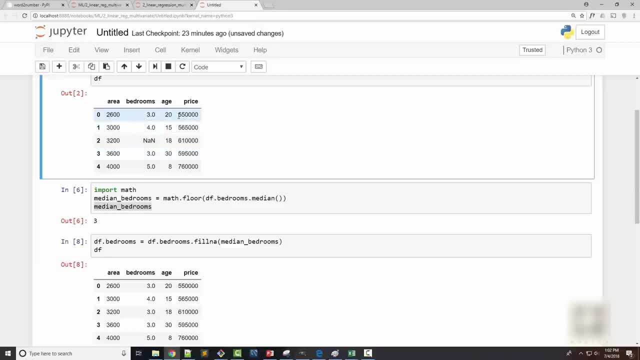 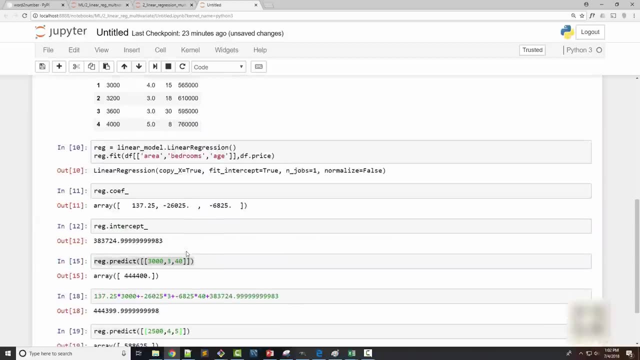 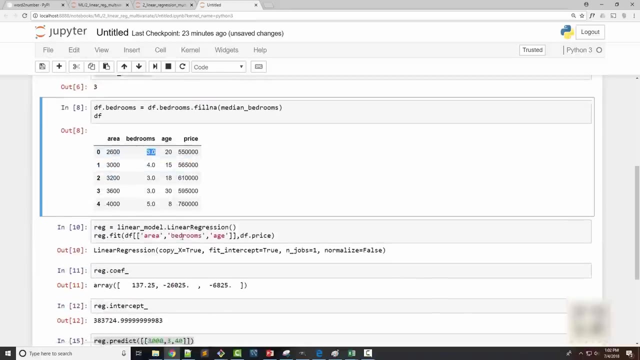 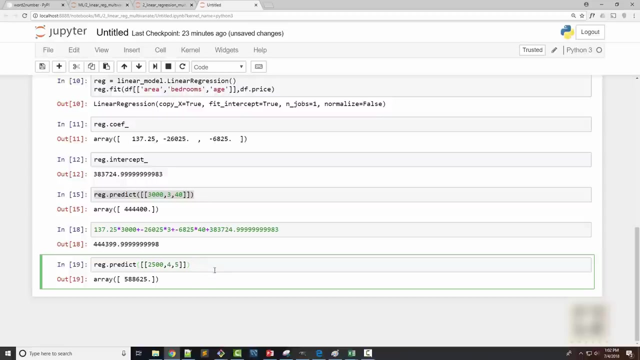 for this home, which was 2600, the price was 550, but this home's price is more, and it is because this home was 20 year old, whereas this home is only five year old and it has one more bedroom. see, this guy had only three bedrooms. so you can see how different factors play a significant role. okay, that's. 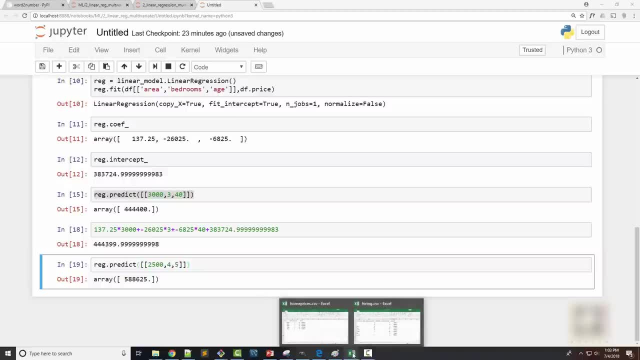 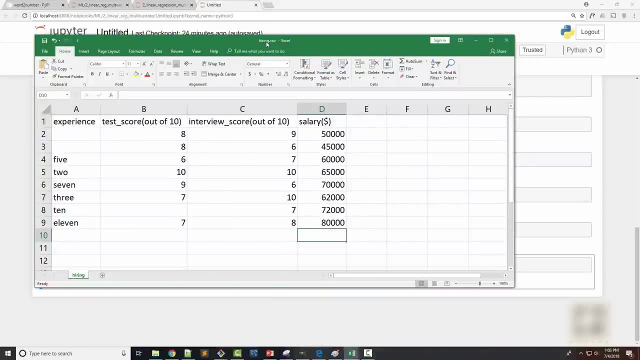 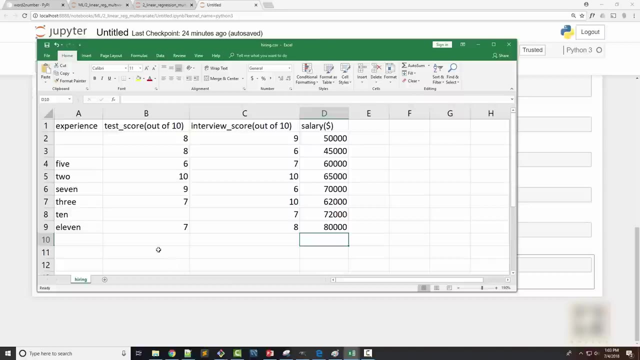 all i had. now we are going to do an exercise, so the exercise is for you guys to practice what you have learned in this tutorial. i have this csv file which contains a hiring data for a firm here based on the experience, the written test score and the personal interview score. 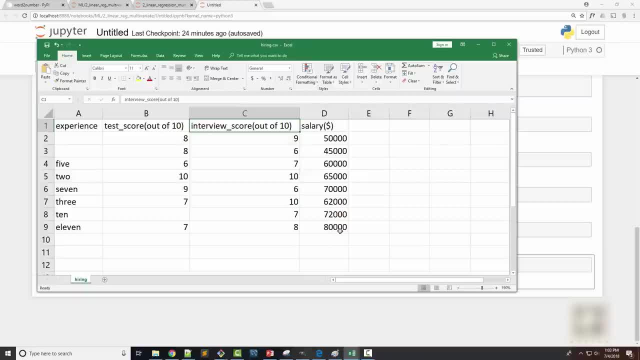 candidate salary is decided and i have some past data. using this data, you have to build a model for your hr department where they can feed in experience data and you have to build a model for your hr department where they can feed in experience data. and you have to build a model for your hr department where they can feed in. 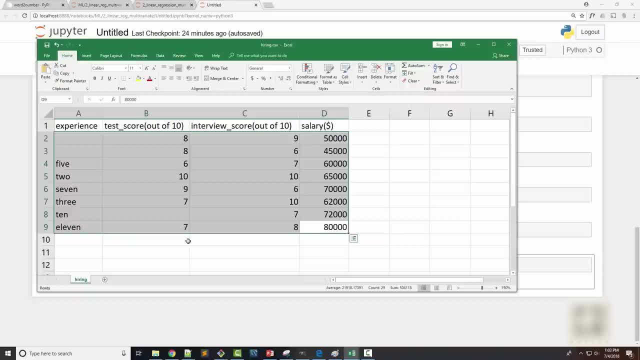 and various scores, and they can get some idea on what kind of salary they need to offer to a candidate. now in this data set, uh, you will find few interesting things. first of all, in experience, these two cells don't have values, so you can just assume them to be zero here. 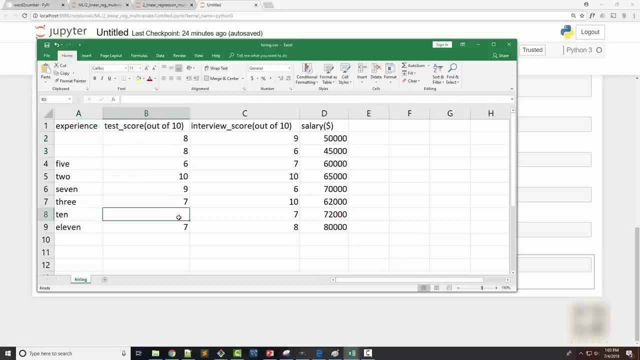 also, there is one data point missing here. you can't, you shouldn't, assume it to be zero. maybe take a median here, all right. and also, usually linear regression models work on numbers, whereas here i have a string. so the experience again it's a number, it's just that. 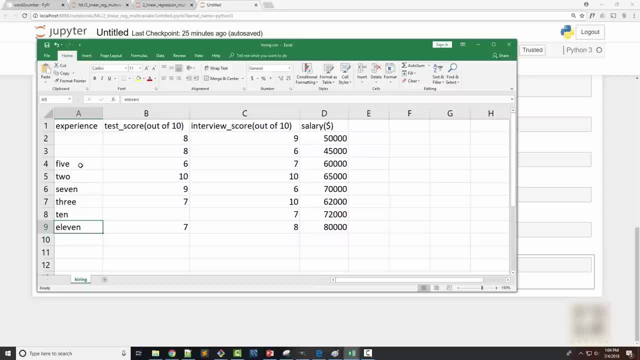 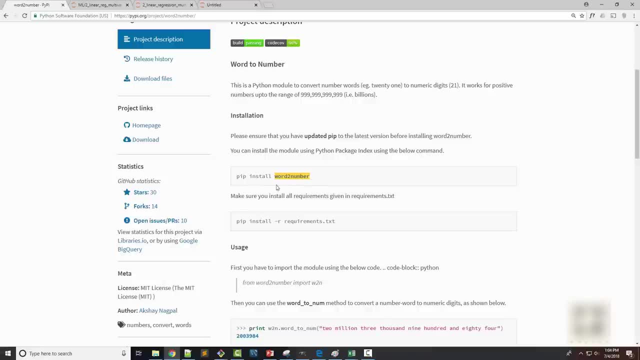 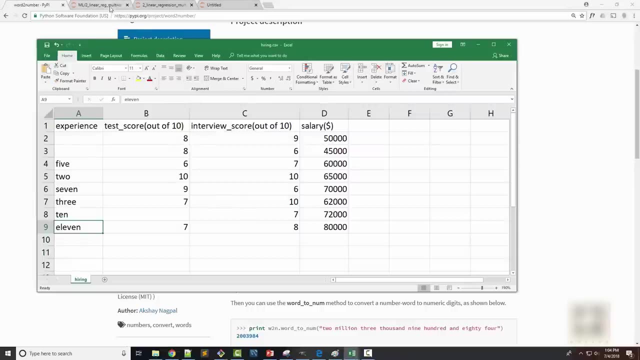 our data set contains word for that particular number. for this, you can use python's word to number module to convert that string into a number, all right, so just do pip, install and use the model, all right, and using this, what you're going to do is, uh, figure out the um. 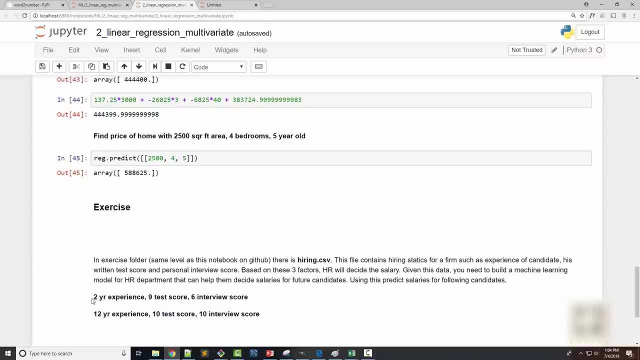 salary for two candidates. uh, who has these statistics? so one candidate has two years experience, scored nine and six into test. second candidate, an excellent guy, 12 years experience, scored 10 out of 10 in both of it. and you have to find out uh recommended salary for.